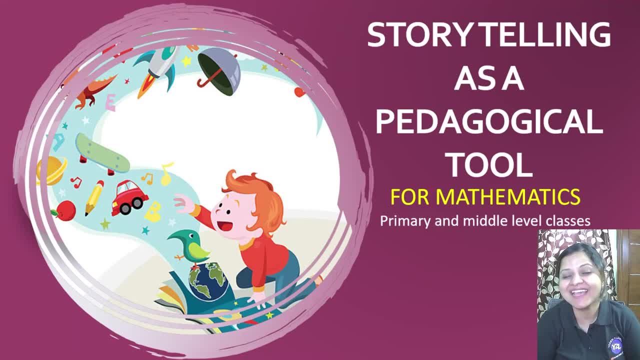 My greetings to all the viewers of Yearn2Learn. And here I am with the second video in the series of storytelling as a pedagogical tool. As I promised that I would come to other subjects also, So in this video I am going to share with you a few examples that how we can use storytelling in mathematics. subject: 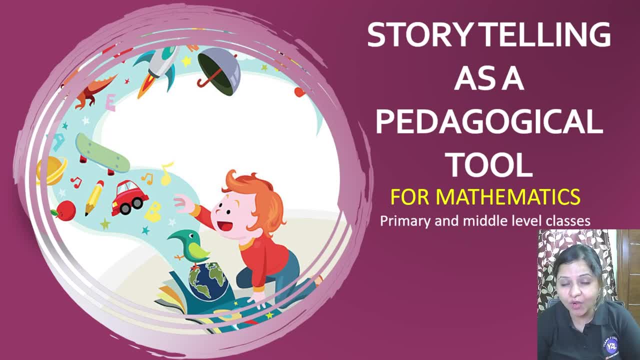 In case you have missed the first video, do watch it. Besides suggestions for using storytelling in English, it possesses the basics of storytelling, So do watch the storytelling video 1.. The link is given in the description box below, And let's begin with how we can use storytelling in mathematics. 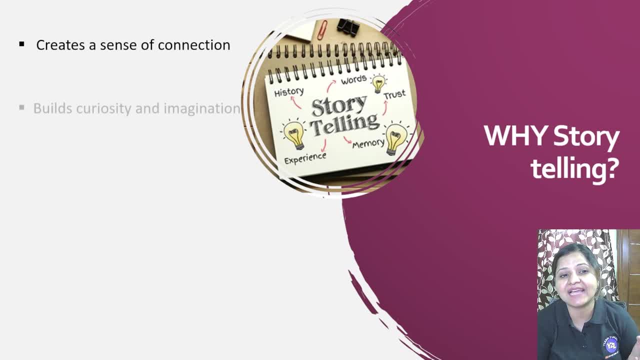 So why storytelling? I explained you earlier also that it can be used in many ways, So let's start with the first video. gives you a sense of connection, it builds curiosity, it helps to remember better- and this is one of the main reasons- and it makes listeners more open towards learning. it conveys 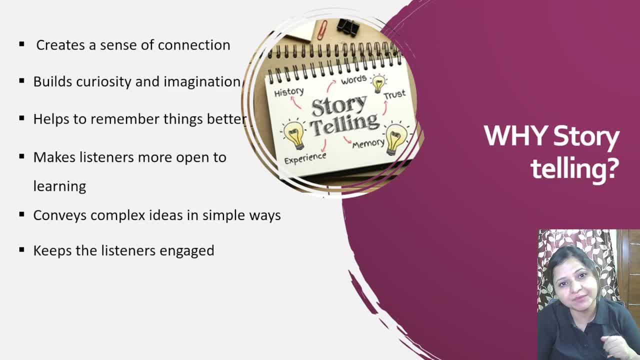 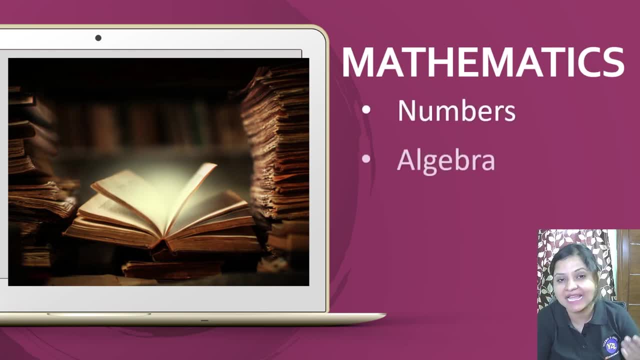 complex ideas in simple ways and, above all, it keeps the listeners engaged. so in mathematics- be it numbers, algebra or geometry- you can use storytelling as a tool. now, those who are good in logic, they love maths. but those who have maths phobia, they tend to not open themselves to learn. 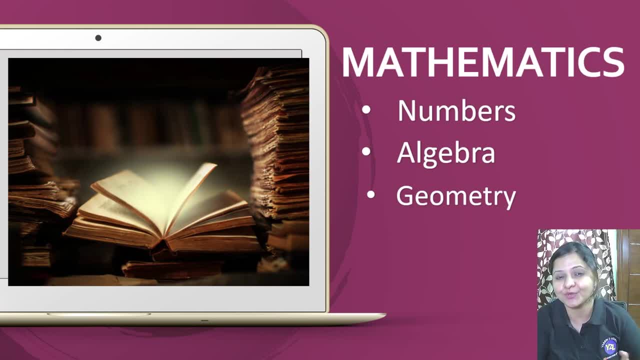 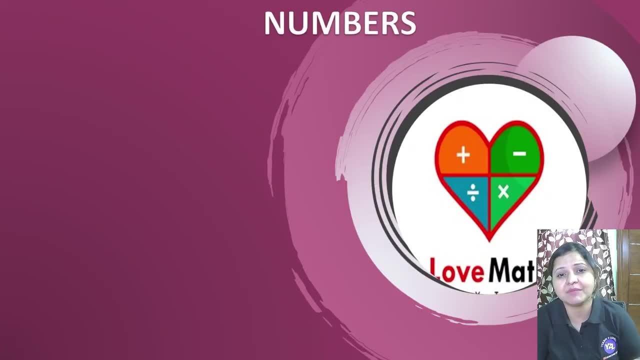 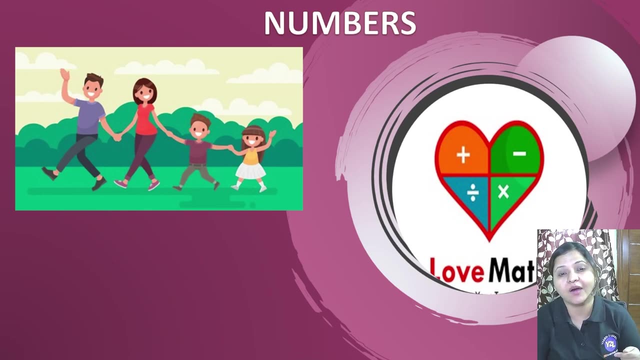 the logic behind various concepts of maths. so what to do? i will begin with examples and let you know how it is effective. so, beginning with numbers, it can be used in primary classes. so here is one story for numbers that you can use for counting, or a predecessor, successor concept, or 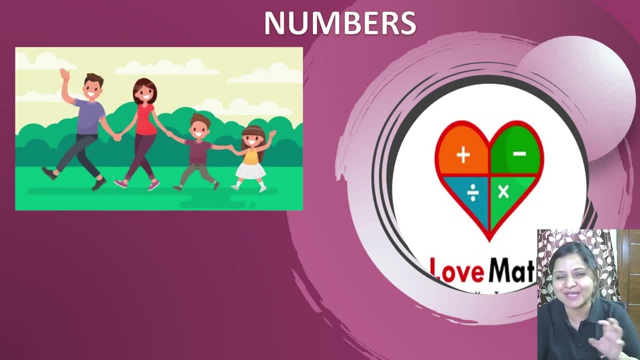 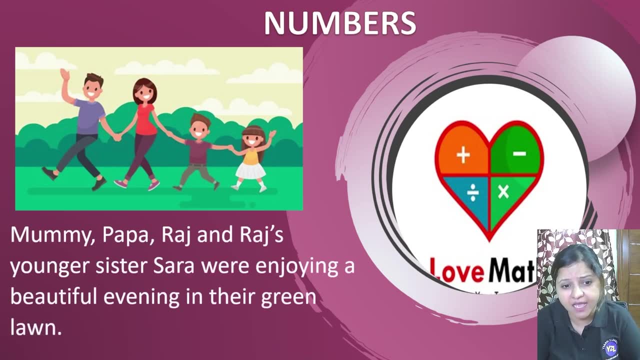 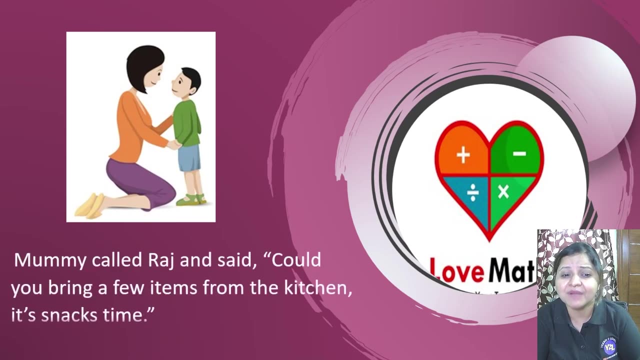 a simple mathematical operations. you can more the story as you want. here is a simple version of it. so mummy, papa, raj and raj's younger sisters sarah were enjoying a beautiful evening in their green lawn. mummy called raj and said: could you bring a few items from the kitchen? it's snacks time. 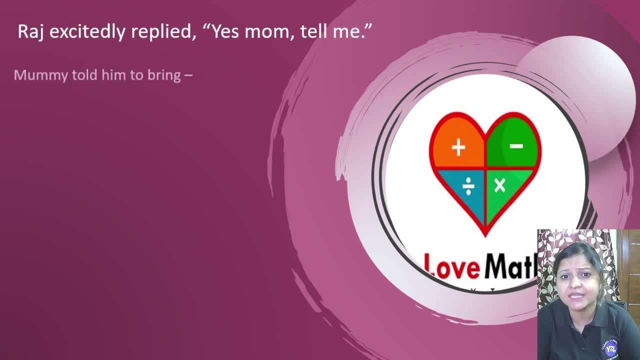 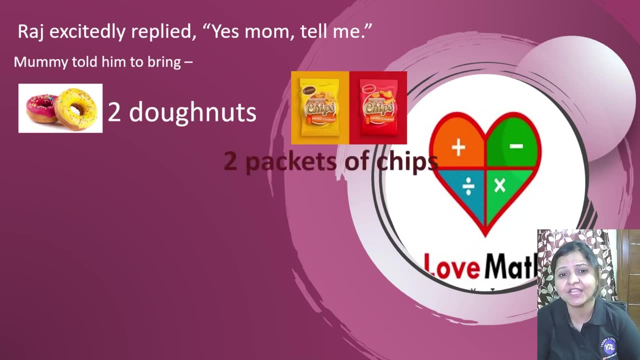 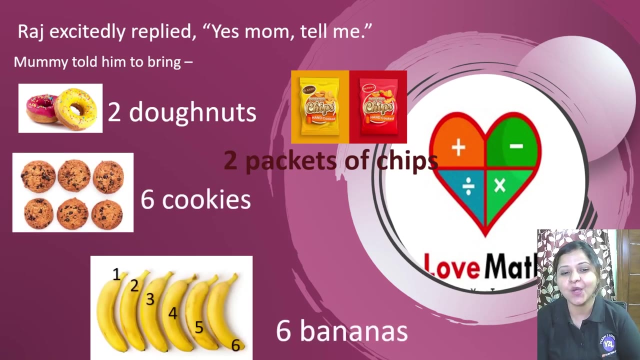 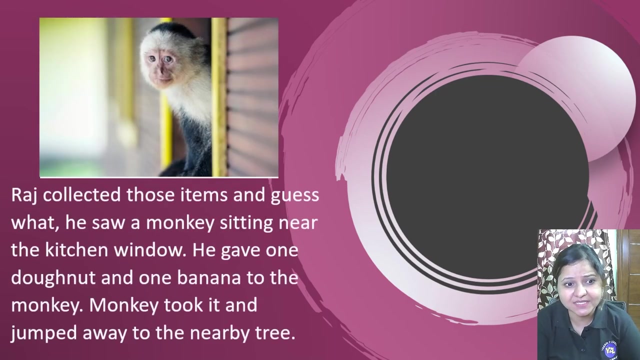 raj excitedly replied: yes, mom, tell me. mummy told him to bring two donuts, two packets of chips, six cookies and one, two, three, four, five, six. come on, say with me one, two, three, four, five and six bananas. raj collected those items and guess what? he saw a monkey sitting near the kitchen window. 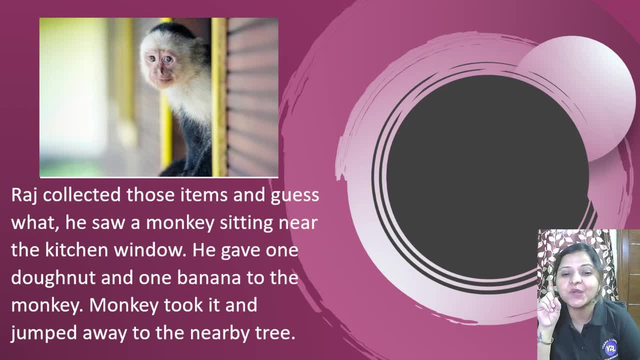 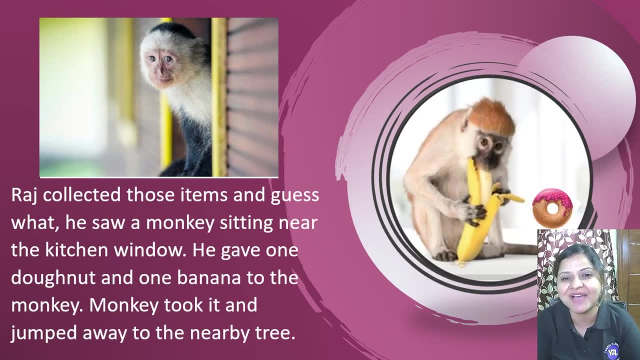 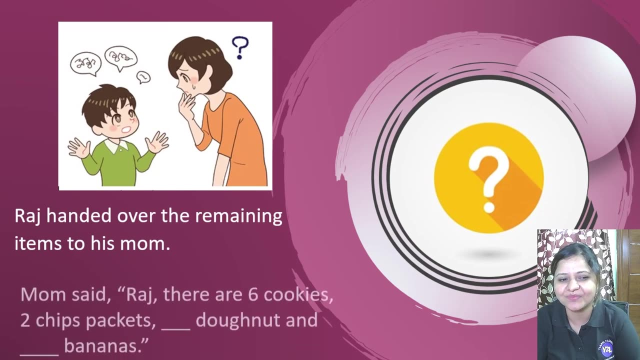 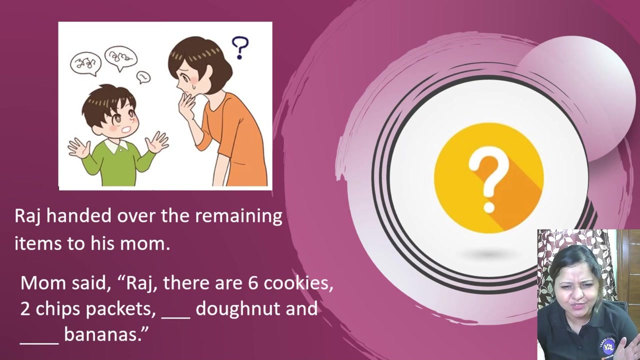 he gave one donut and one banana to the monkey. monkey took it and jumped away to the nearby tree. raj handed over the remaining items to his mom. mom said raj, there are a few items only. do I have to take them out of the kitchen? There are six cookies, two chips, packets dashed donut and dashed bananas. 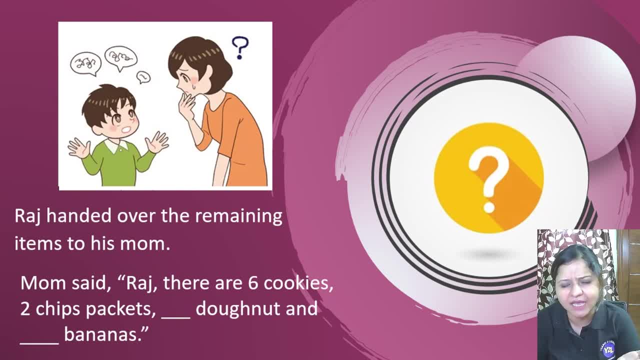 Hey children, can you guess how many donuts and how many bananas? Because what mother said? it was not same in number. Oh yes, Raj gave something to monkey also. So this is how you can encourage students to think about it. They will recall that there were two donuts. 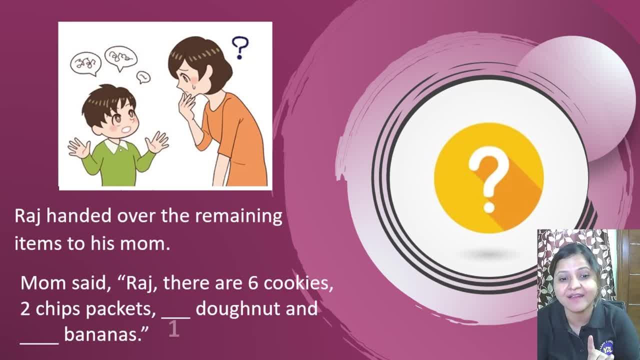 One was given to monkey. So how many donuts should be there? One donut, and there were in all six bananas, and one banana was given to the monkey by Raj. So how many bananas? Five bananas. So this is basically minus one concept. 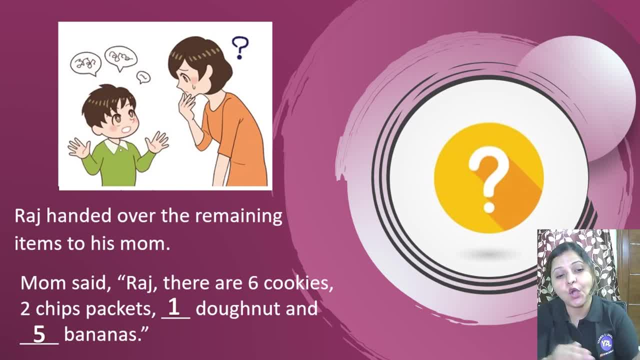 You can bring that in, or you can keep it simply to counting, or you can bring it to addition How many total items Raj gave to the mother. So this is more like a story sum, but visual and with a theme Students would read. They would relate to it better and would be excited to do this simple number maths here. 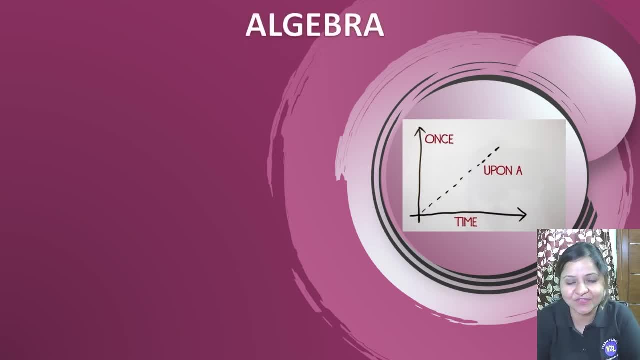 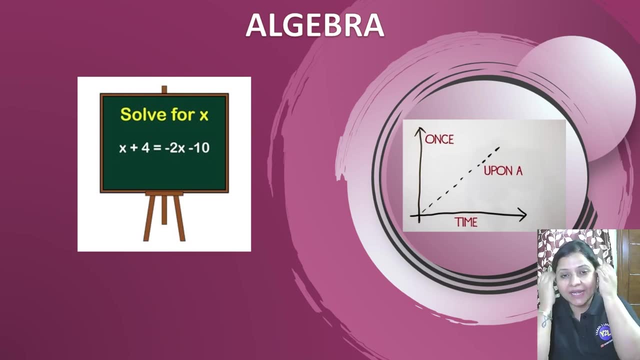 Coming to my second example, My second example is of algebra and I am taking a simple equation here: Solve for X. Now, when I take that equation, maths teacher, I'm already folding my hands right. So please do not look for the logic right away, because it is storytelling. 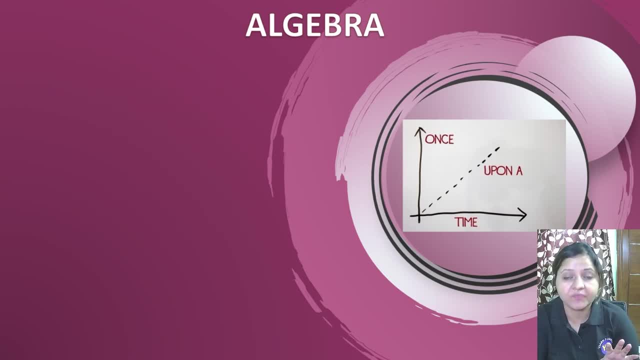 I tell you where this storytelling is. I tell you where this storytelling method is effective. This method is effective where students are not open towards maths or do not enjoy mathematics or they have phobia, maths phobia. So what you can do is you can use storytelling as a powerful tool to introduce the concept, to let them know and be aware of the rule. 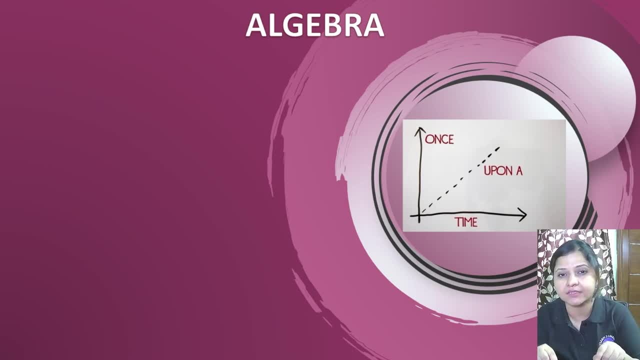 And once they are thorough with that, through storytelling method, you can bring the logic in later. So this is how you can do. This is more like a trick, but it is very successful. I have already tried it with students. So here I'm taking an equation: 2X minus 3 equals to 7.. 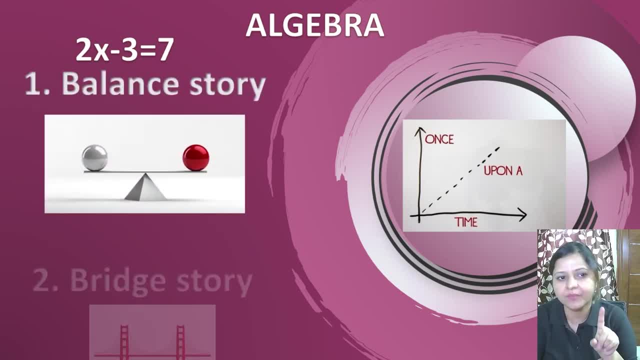 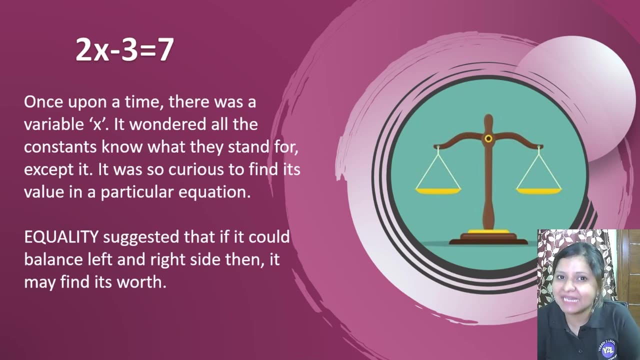 I'll give you two stories on this. One is the balance story and the second is the bridge story. I'm sure, being maths teacher, you will be able to find the logic in it. Let's begin with the first one. Once upon a time there was a variable X. 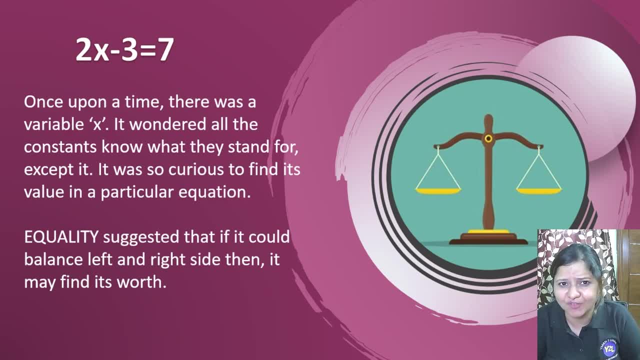 It wondered. all the constants know what they stand for except it. It was so curious to find its value in a particular equation. Equality suggested that if it could balance left and right, then it may find its worth. Oh, balancing left and right. 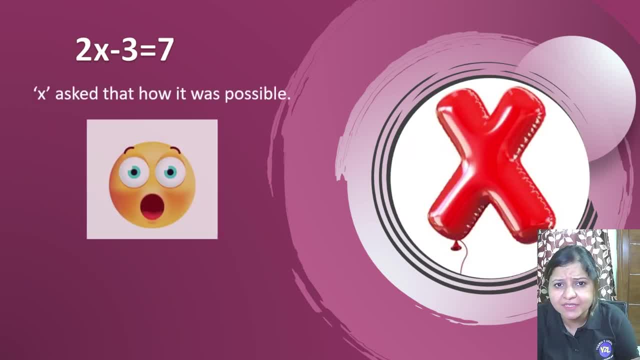 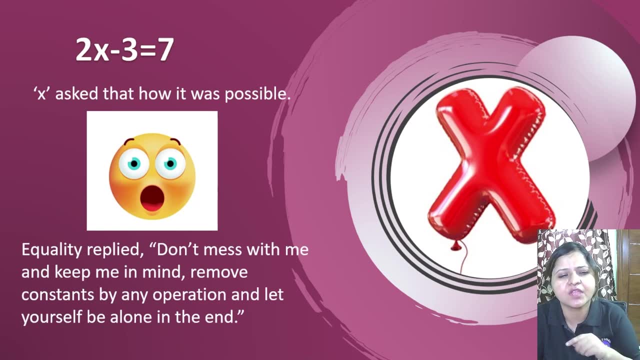 X are. It was just that how it was possible. equality replied: don't mess with me and keep me in mind. Remove constants by any operation and let yourself be alone in the end. So equality told that use any operation and eliminate the constants and be alone in the end. 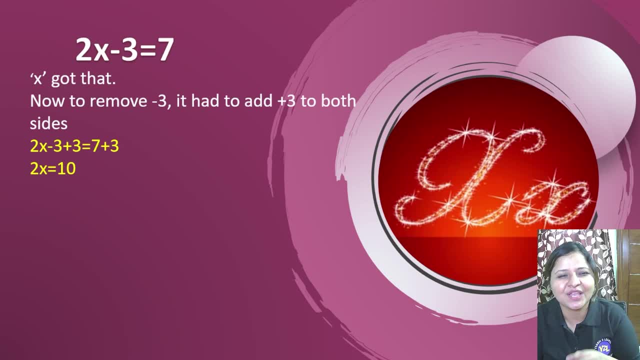 And you would find your worth. X got that. Now, to remove minus three, It had to add plus three to both sides, So two X minus three plus three and seven plus three. So two X would give you ten. And then to remove two, it had to simply divide both sides by two so that equality could be maintained. 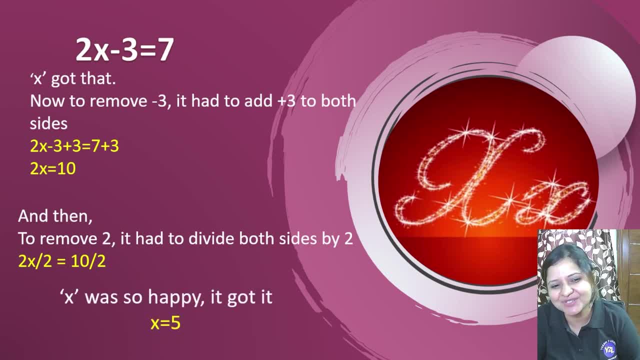 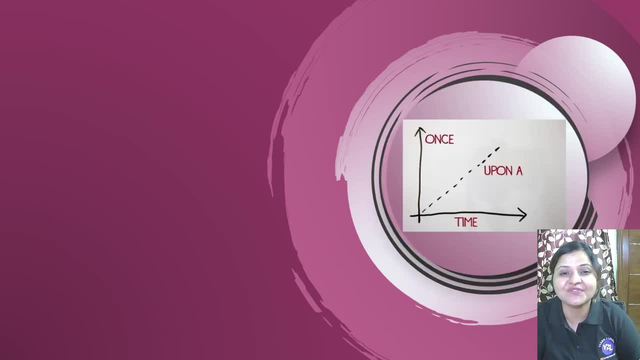 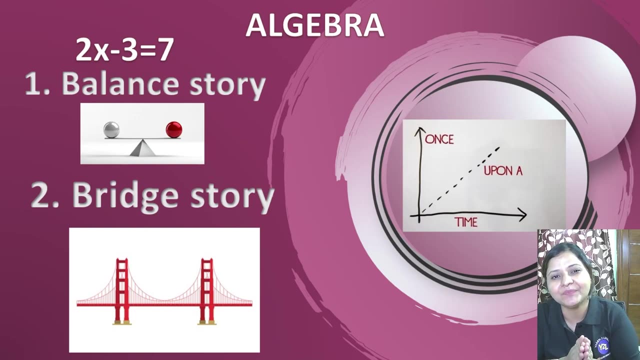 So two X by two equals ten by two X was so happy it got it- X equals five. So this was the first story. So, as I said that I'm going to take the two stories in it, I like the second version better to. for the same equation, same concept: the bridge story. 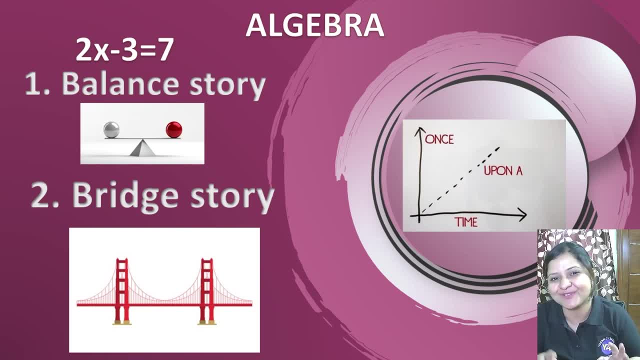 Now this is more like a story and less like the previous story, which sounded like logic. Now how I'll tell you. I'm again going to repeat that this is maths. This is all built by logic, But sometimes we need to bring the fantasy factor in. 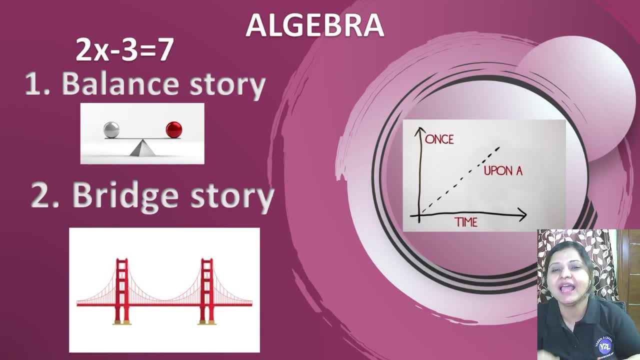 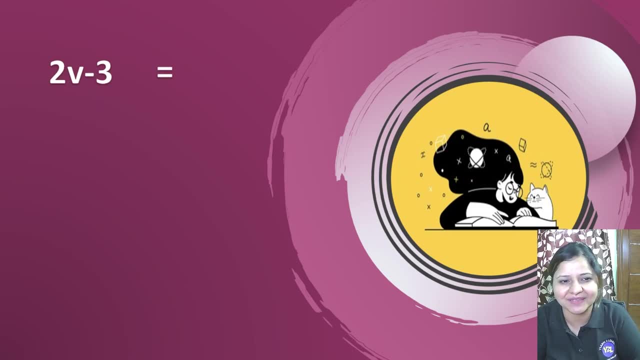 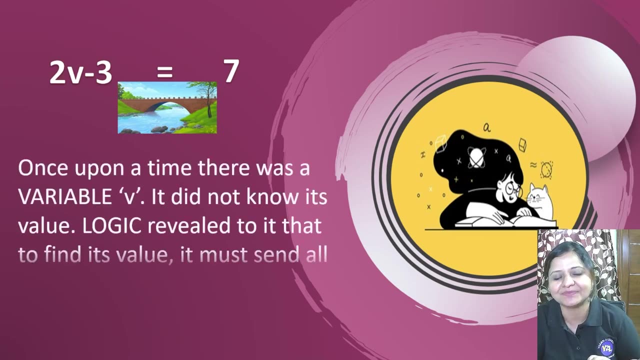 So that students get the concept, They learn the rule, and then we can explain them the logic once they are comfortable with it. Let's begin with the second story on the same thing. So, as I said, it was a bridge story. Now bridge is having very important role here. 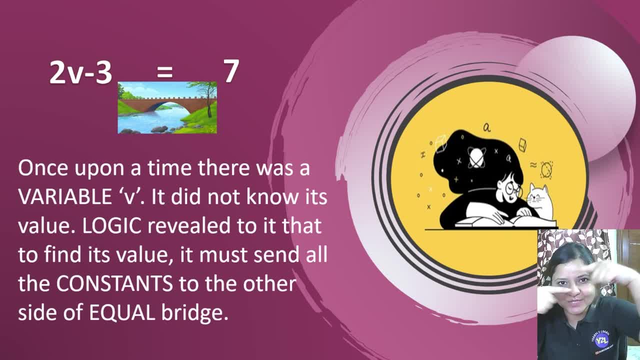 So what we are doing is we are considering equal to sign as a bridge. Once upon a time there was a variable V. It did not know its value. Logic reveals to it that to find its value, it must send all the constants to the other side of equal bridge. 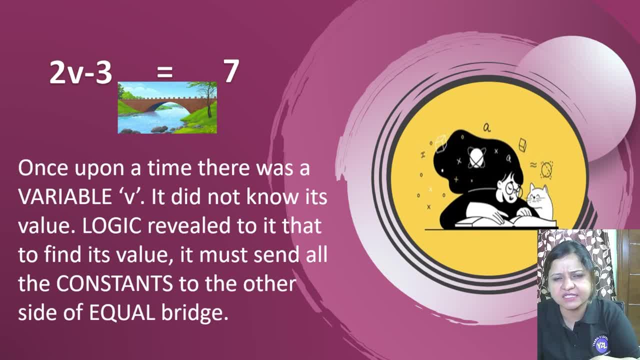 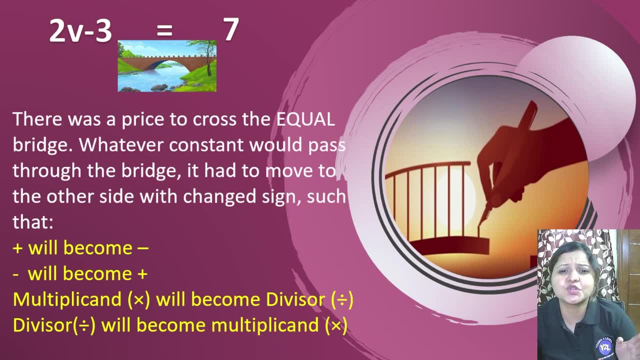 So equal bridge: send all the constants to the other side. Then only we can find its value. There was a price to cross the equal bridge. Whatever constant would pass through the bridge, It had to move to the other side With changed sign. 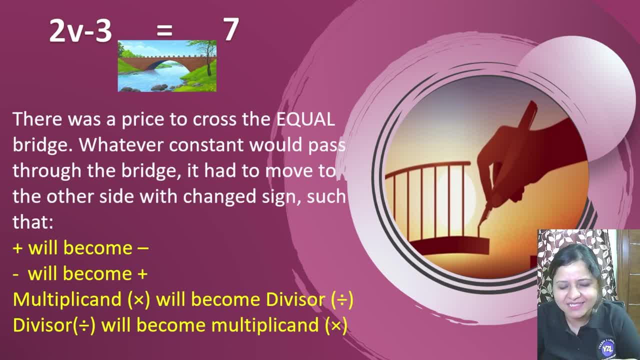 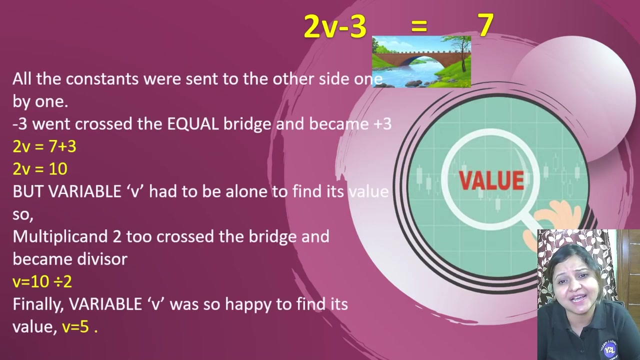 Such that plus will become minus, Minus will become plus, Multiplicant will become divisor And divisor will become multiplicant. So this opposite had to happen. It is more like a toll that you have to pay to cross that bridge. All the constants were sent to the other side, one by one. 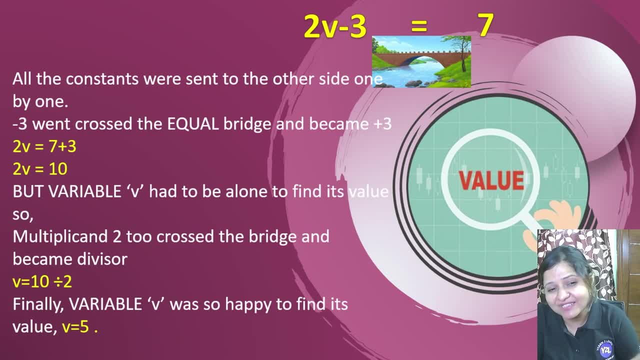 First of all, minus 3 went. It crossed the equal bridge And became plus 3 on the other side, And that's how we got 2V equals to 10. But variable V had to be alone and find its value. Still, 2 was there with it.